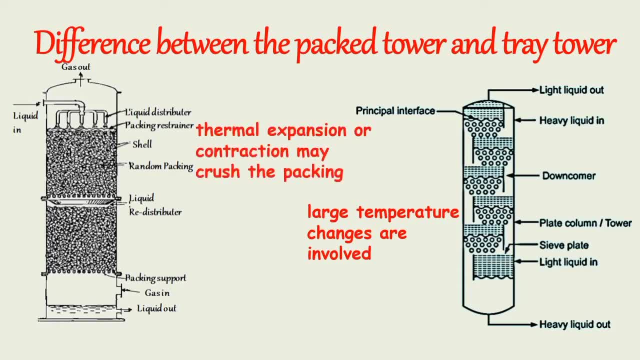 Thermal expansion or contraction of the equipment component may crush the packing, As the pressure drop through a packed tower is usually low, Which makes the packed tower particularly desirable for vacuum distillation operations. Packed towers may be more economical Than plate towers When highly corrosive fluids are to be handled. 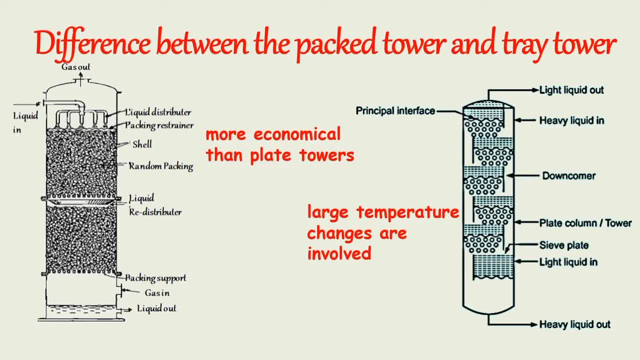 Because of corrosion resistant ceramic or plastic packings. Plate columns operate over a wide range of liquid flow rates without flooding. High values of liquid gas ratio are best handled in packed towers. In a packed tower, difficulties arise in the dispersion of liquid, Hence a plate tower is more reliable. 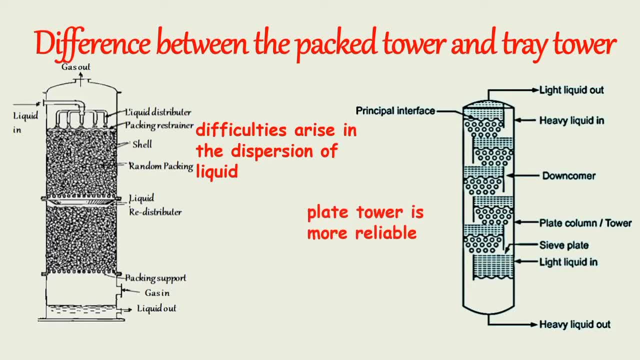 And needs fewer safety factors at the low liquid to gas mass velocity ratios In plate columns. By repeatedly mixing and separating provide More positive contact between fluid phases, Whereas packed columns may lead to back mixing or bypassing. Side streams are very easily taken out from plate towers. 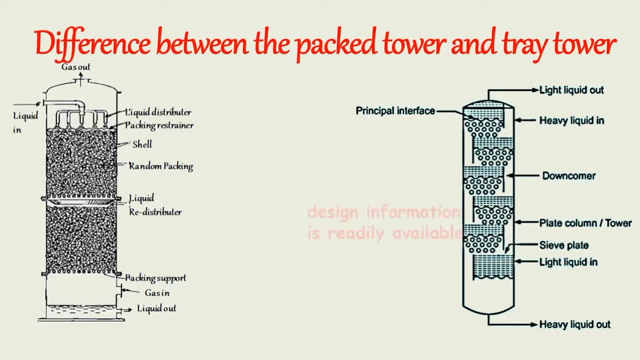 For plate towers, Design information is generally more than required And information is generally more readily available And it is more reliable than it is for packed towers. Plate towers should be preferred When liquid mixtures containing dispersed solids are to be handled, As cleaning the plate is very easy. 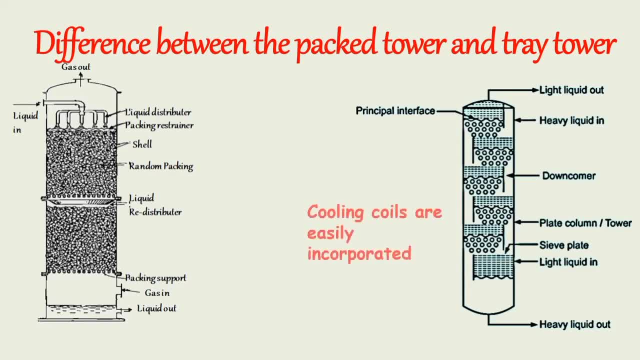 Plate towers are preferred Whenever an intermediate cooling arrangement is required To remove the heat of a solution or reaction. Cooling coils are easily incorporated into plate towers For liquids having a tendency to form. Packed towers are usually preferred For a given duty. 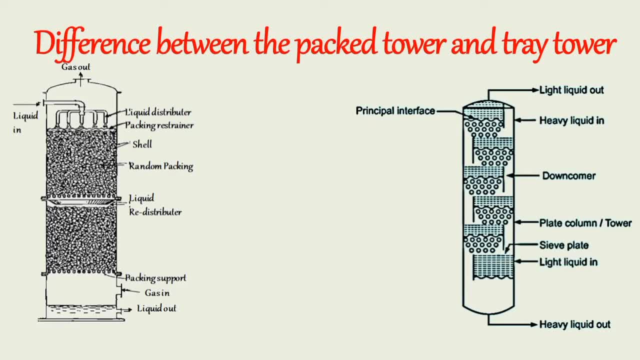 The total weight of a dry plate tower Is normally less than the weight of a packed tower, But the weight of both towers is approximately the same If the liquid the hold up in the plate tower during the operation is taken into account For a column diameter of more than 1200 mm.